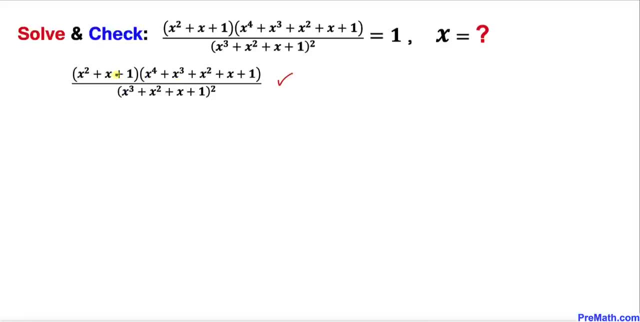 this is a huge polynomial, So it will be really hard to multiply and then divide. So therefore, we have to be creative and think outside the box. So, therefore, I am going to multiply the top and the bottom by 1 minus x- whole square, and at the same time I'm going to 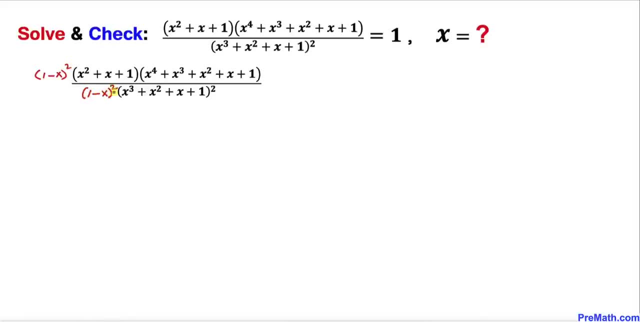 divide by 1 minus x whole square as well. And now let's focus on this top part: 1 minus x whole square. This could also be written as 1 minus x times 1 minus x, isn't it? And in this next step, I: 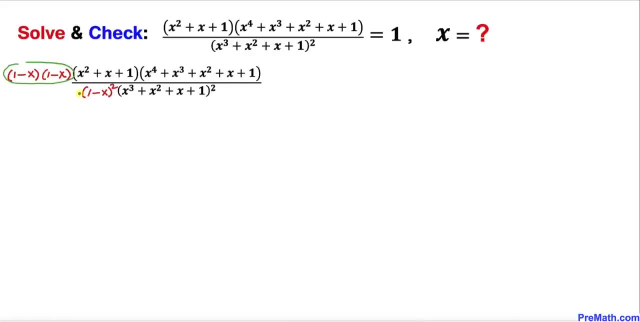 wrote down 1 minus x times 1 minus x, And now we are going to rearrange this: 1 minus x and 1 minus x. I'm going to put 1 minus x, 1 with this one and the other with this polynomial. So therefore I can. 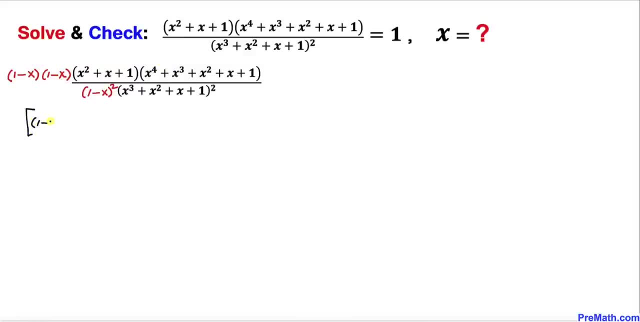 write 1 with 1 minus x times. I'm going to put this polynomial first: x square plus x plus 1.. And let's write down the other one: 1 minus x times. this other polynomial which is divided by this denominator could be written as I can write like this thing: 1 minus x times x power, 3 plus x square plus x plus. 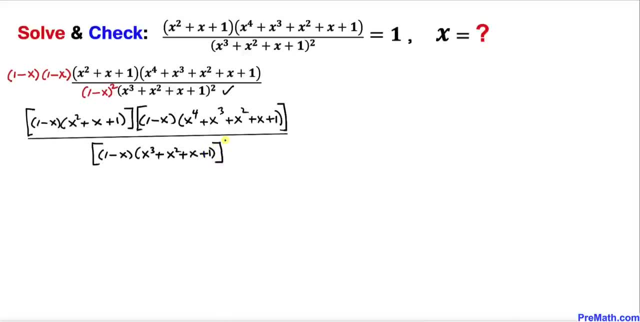 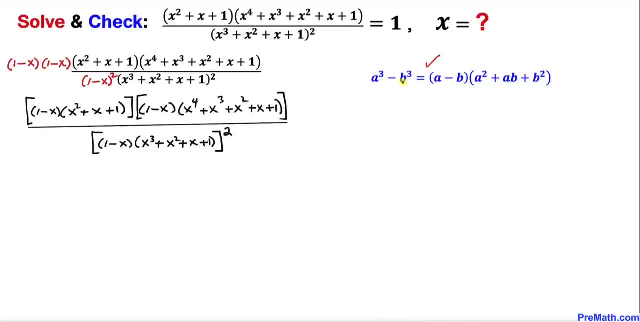 1 and that's bracket closed. and then I'm going to put down whole square. And now let's recall this famous identity: a cube minus b cube. and if I suppose that a equals to 1 and b equals to x, then we can see that this is going to become 1 minus x cube. 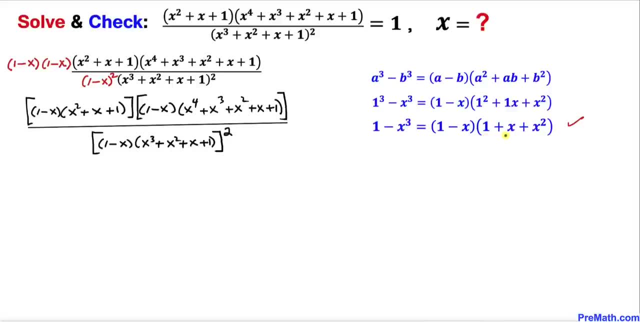 equals to 1 minus x times 1 plus x plus x square. And likewise, if we extend this formula, we can write 1 minus x power 4 equal to 1 minus x times 1 plus x plus x, 2 plus x power 3, and if you are wondering how that is possible, so let me go. 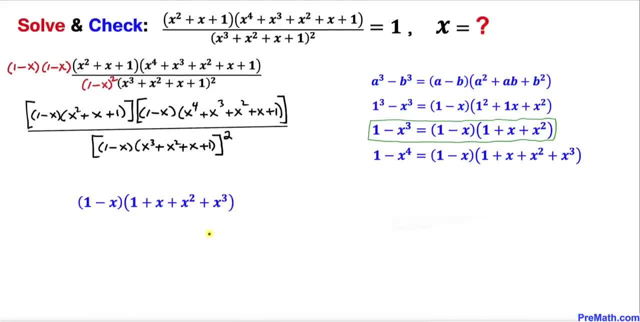 ahead and show you a justification. and here I have copied down the right hand side of this equation. and let's go ahead and multiply these two polynomials. and here I have distributed this one with all of them in the Wolfram admiration graph. this one, and that's what we got. and then I distribute this negative x all the way to this one. 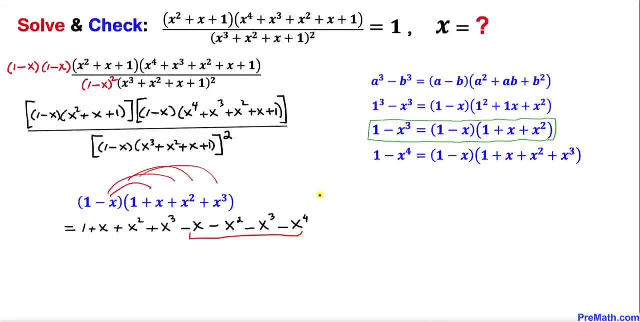 and I got this part as well, and now we can see that this x and minus x is gone. x square minus x square is gone. x cube and minus x cube cancel each other out. so we ended up with only 1 minus x power 4, and that's what it's supposed to be, and likewise we can extend this formula to the next. 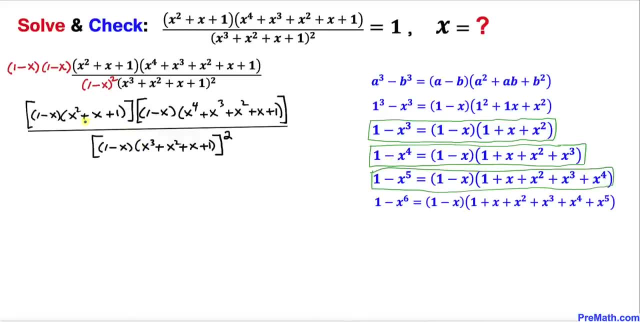 level, as you can see. and now let's revert our attention back to our this original problem over here. let's focus on this part. we can see that this is equal to 1 minus x cube, so I'm going to replace this one by 1 minus x power 3. and now like: 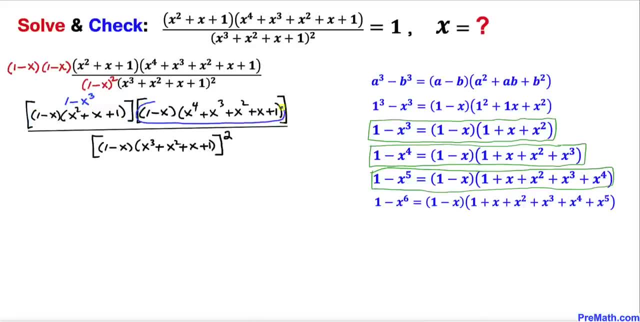 let's focus on this part in this bracket. this is same as this one, so this is equal to 1 minus x power 5. so therefore, I'm going to replace this one by 1 minus x power 5, and likewise, let's focus on this denominator, this part inside this bracket. this is same as this one, so this is equal to 1. 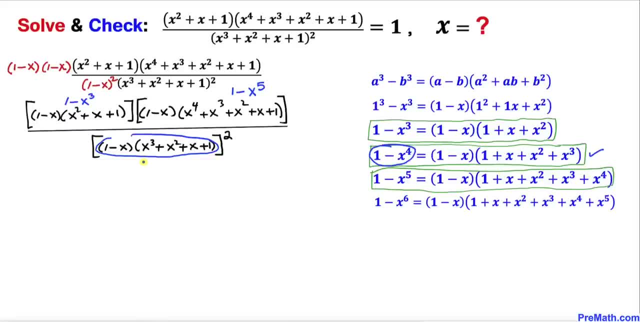 minus x power 4. so therefore, I'm going to replace this one by 1 minus x power 4. so therefore, our this expression could be written as 1 minus x power 3 times 1 minus x power 5, divided by this one: 1 minus x power 4, whole square. and in this next step we 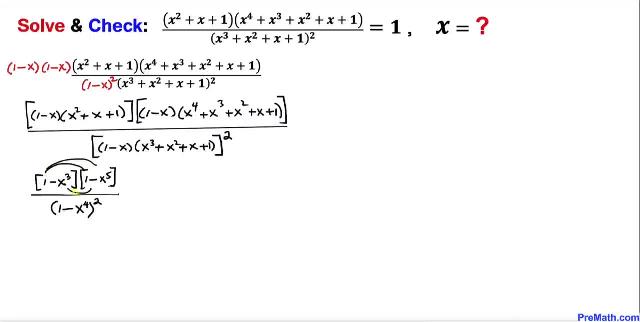 are going to do the double distribution. we're going to use this rainbow method, so that is going to give us 1 minus x power, 5 minus x power 3 plus. when we multiply this thing, that's going to give us x power 8 divided by. and now let's recall this famous identity: a minus b, whole square. 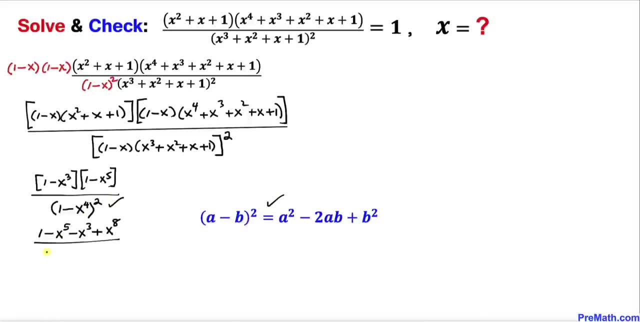 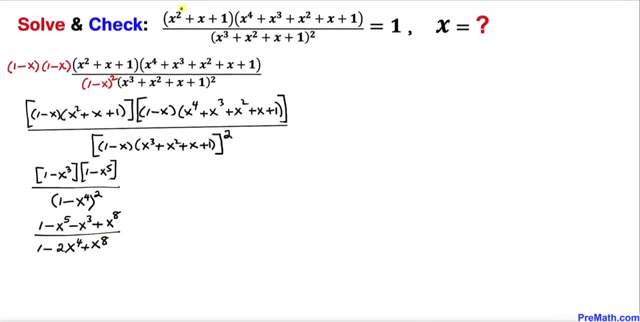 so we are going to apply on this one. so that is going to give us 1 minus 2 x power 4, then plus x power 4. whole square is going to make is x power 8, and now we can see that this whole left hand. 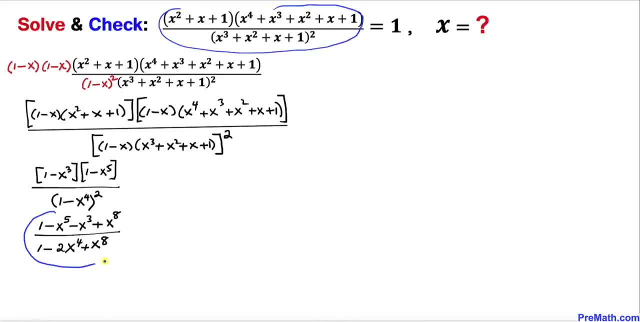 side of this equation has been simplified to this one, and since this left hand side is equal to 1, so I can write this thing equal to 1 as well. now this one could be written as 1 divided by 1, and let's go ahead and. 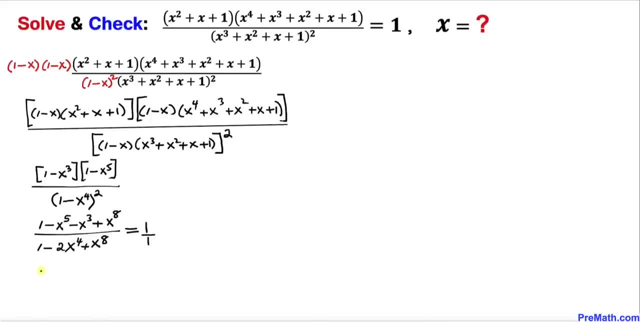 cross multiply on both sides. so this could be written as 1 minus x power, 5 minus x power, 3 plus x power equals to: on the right hand side, that's going to be 1 minus 2x power, 4 plus x power 8, and now we can see that this x power 8 and x power 8 is gone and this: 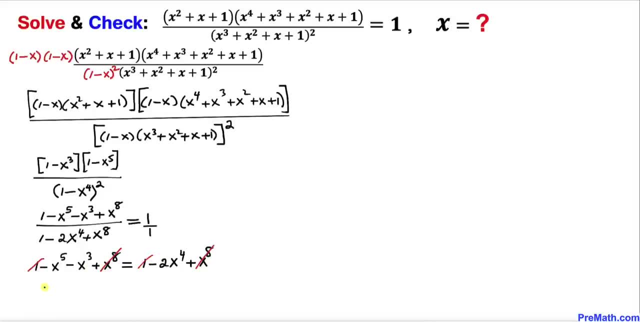 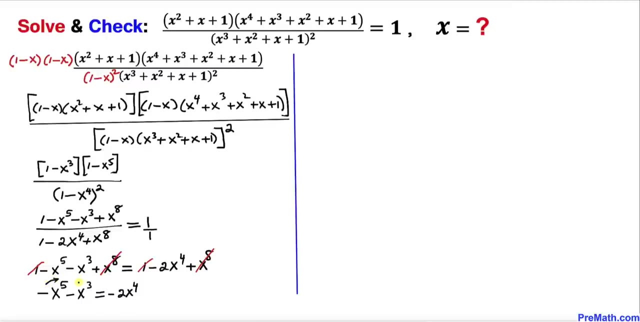 1, and 1 is gone as well, so we are left with simply negative x power 5 minus x power 3, equal to negative 2x power 4. and now let's go ahead and move everything on the other side, so we are going to get x power 3 minus 2x power 4. 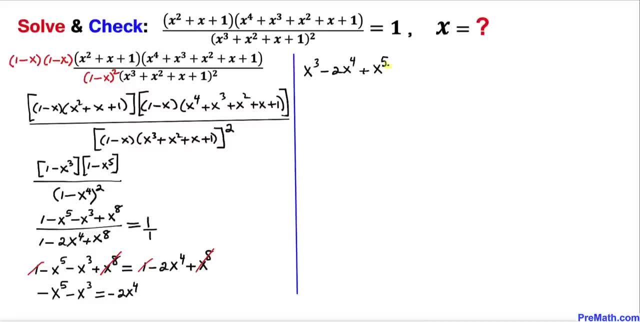 plus x power 5, equal to 0, and here we can see that x power 3 is in common, so I can factor that one out. so we ended up with 1 minus 2x plus x square, equal to 0, and this part is same as 1 minus x whole.